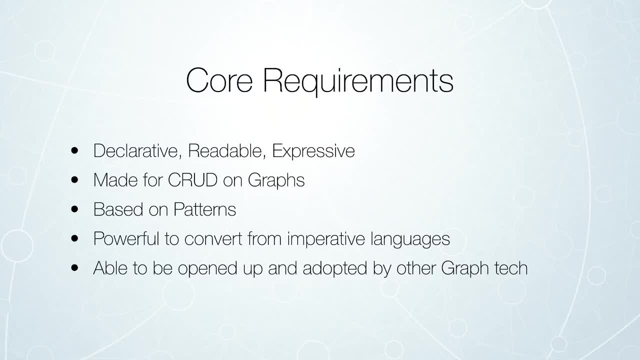 more popular by you know different communities, So we really wanted a declarative query language very similar to how many developers use SQL when interacting with tables. We wanted a similar declarative language for graphs. We wanted it to be able to do all CRUD operations: create, read. 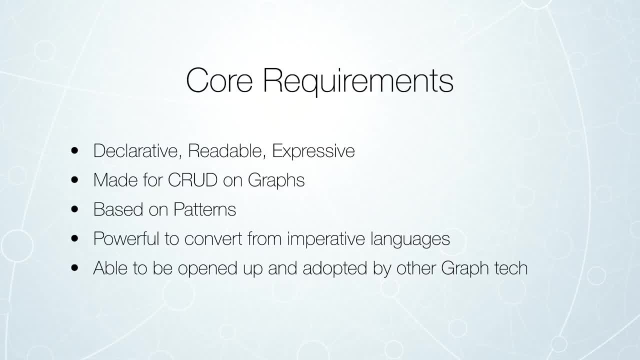 update, delete all the main operations, not just be a querying language. We also wanted to base it on patterns- the core patterns that you're looking for in a graph, And we wanted to make it really powerful so that you could actually convert people from using the. 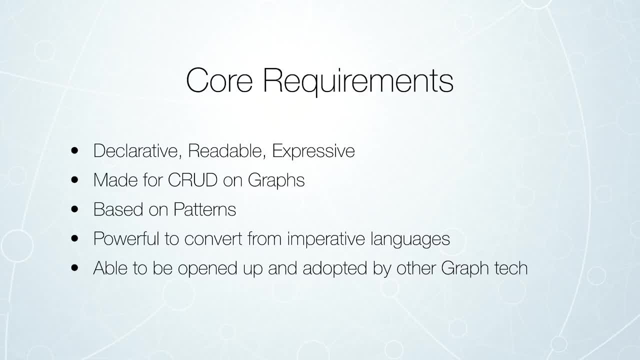 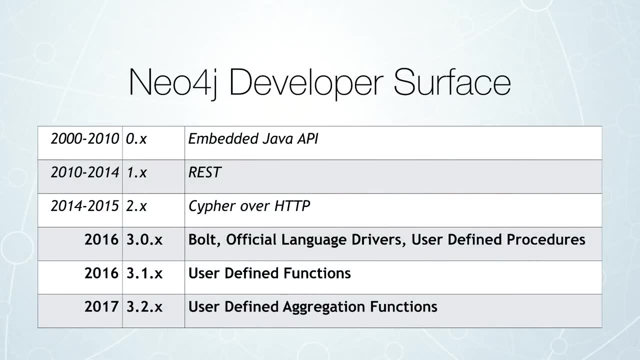 more imperative languages over to this declarative language And we wanted to allow it to be opened up and adopted by other graph technology. So, in order to do this, we invented the next set of developer surface for Neo4j, and that was Cypher over HGP And that was Cypher over HGP. 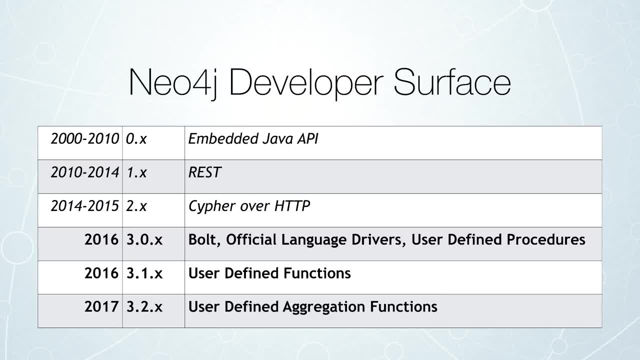 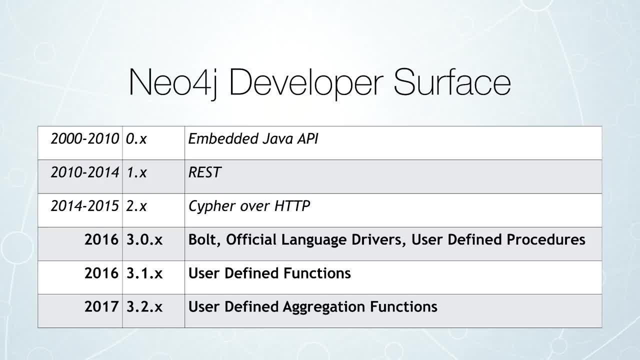 this declarative language in order to access it. And then, as we advanced on into the 3.0,, 3.1, 3.2 series of Neo4j, we also launched the Bolt protocol, a binary protocol. that makes it much. 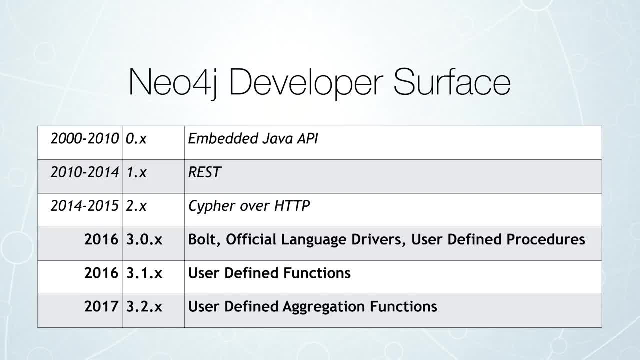 more type safe to interact with Neo4j, And we also launched the Bolt protocol, a binary protocol that makes it much more type safe to interact with Neo4j And provides a series of official language drivers such as Java, NET, Python and JavaScript, And user defined procedures. 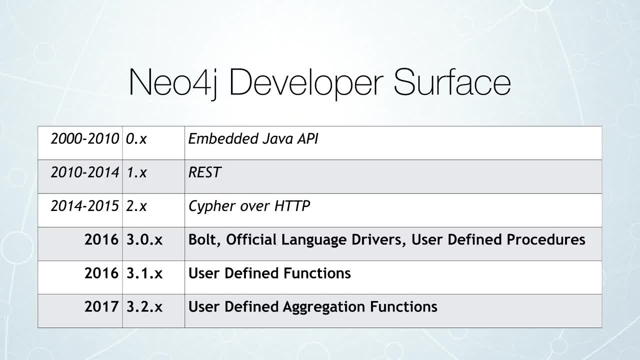 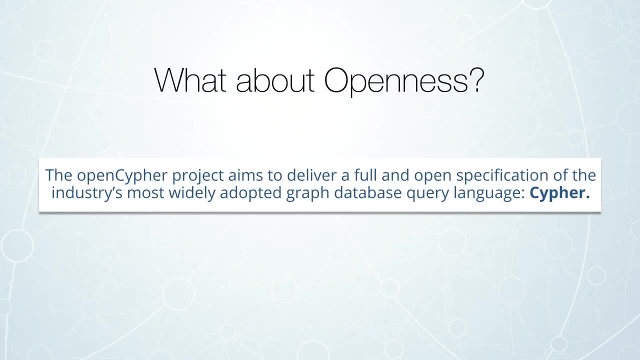 and functions so that you could still do those interactions with the Java API if you want to, but call them from within Cypher. All of the procedures and functions can be called from within Cypher, And that was very important to us From an openness perspective. we wanted 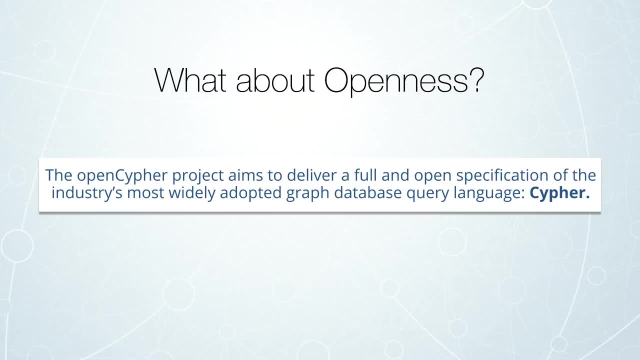 to release Cypher under the OpenCypher project. OpenCypher aims to deliver a full and open specification of the industry's most widely adopted graph database query language: Cypher. You can visit OpenCypherorg to find out more about the OpenCypher project and other databases. 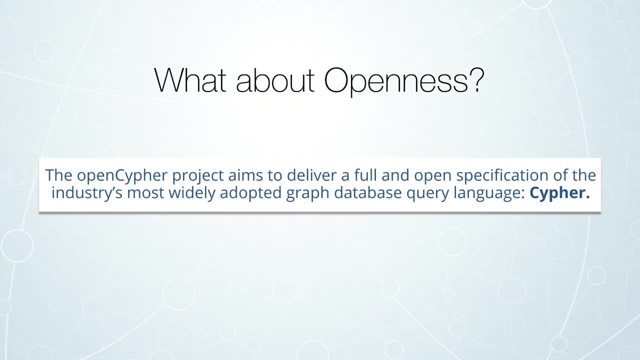 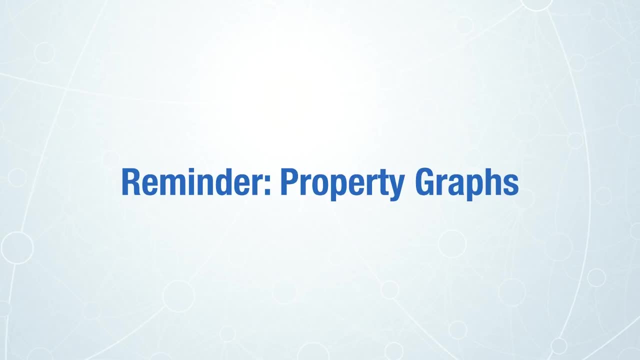 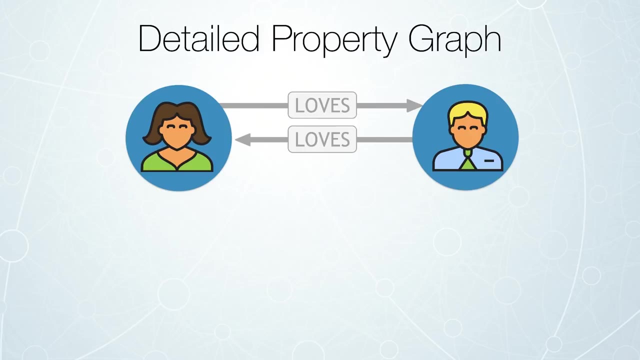 such as SAP HANA, which have adopted the Cypher technology. Now, as I review Cypher, I'm going to give you a reminder and a little bit of a recap of what property graphs are. A property graph has a concept of a node and a relationship and properties on both those nodes and relationships. 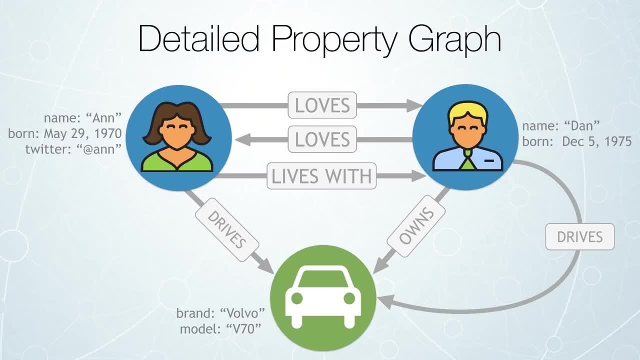 So in the case here, we have Ann who loves Dan, Dan who loves Ann, back and lives with Dan, And Ann drives a car- I think for both nodes enough information for two different possibilities, And I also- which is owned by Dan. Dan also drives that same car, So you can see here that 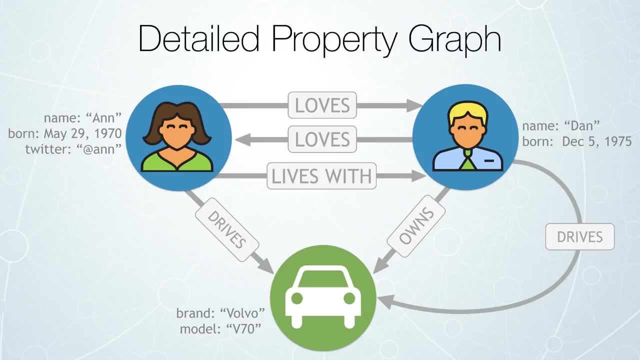 it's very easy to read this graph even without having a full understanding of graph databases and cipher and property graphs. It's really easy to read what's happening here- And this is an important characteristic of Neo4j and graph databases- is the whiteboard model, is the physical model. We try to reduce the. 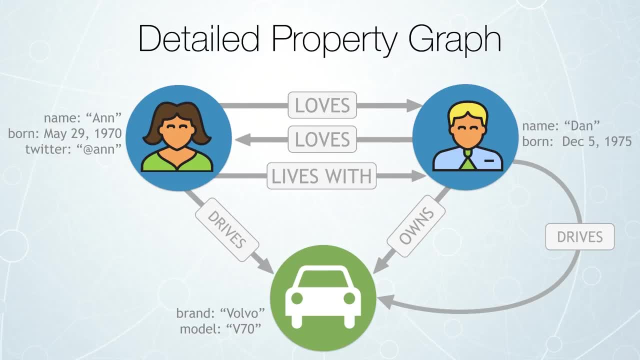 number of translations between the business owner and the developer and the underlying system which is executing and storing data. So we create the nodes and relationships in the underlying datastore as sort of the nouns and the verbs and create the properties on the nodes as sort of the adjectives and the. 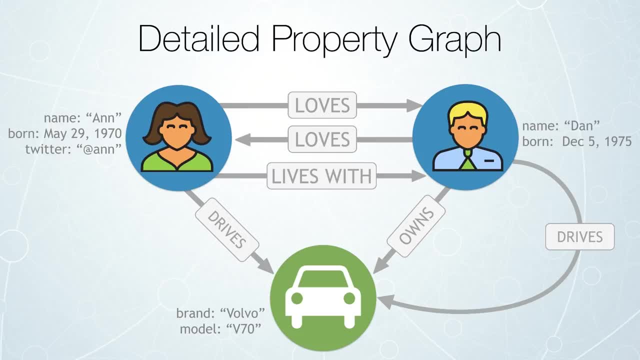 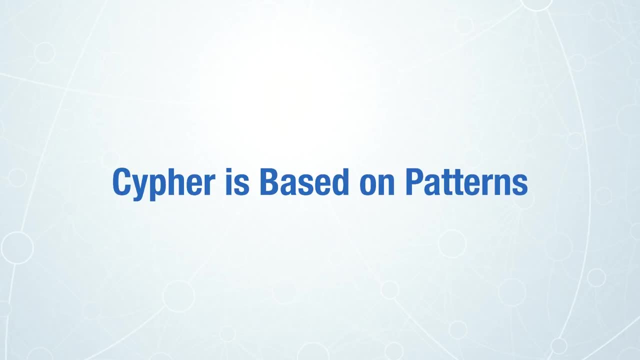 properties, on the relationships, as sort of the adverbs. So that's the Neo4j, That's the, the overview or recap of the property. graph model Cipher as a query language is based off of patterns. It's about creating patterns in a graph. 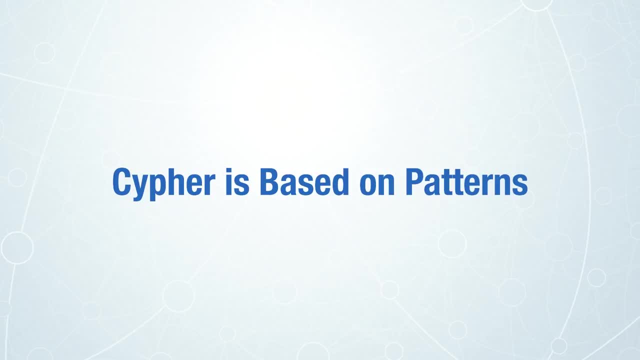 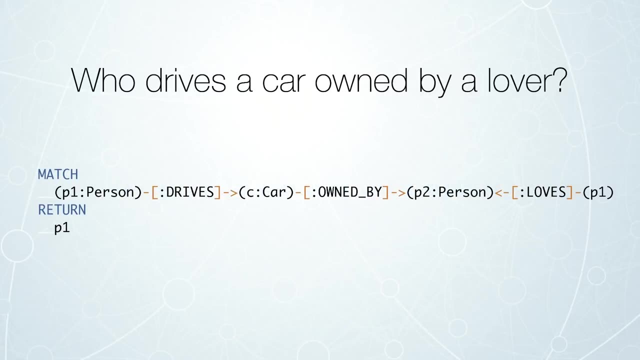 patterns of nodes and relationships, and then it's about finding those patterns when you're doing your queries. So here's an example of one pattern that you might specify. It's a fairly complex pattern but very easy to read and understand and even code in. 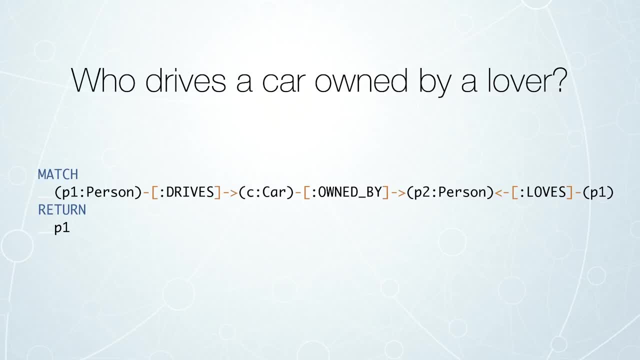 Cypher. So we want to find out who drives a car that is owned by a lover And in this case, meet just right at out match a person who drives a car which is owned by another person and the original person loves that other person. 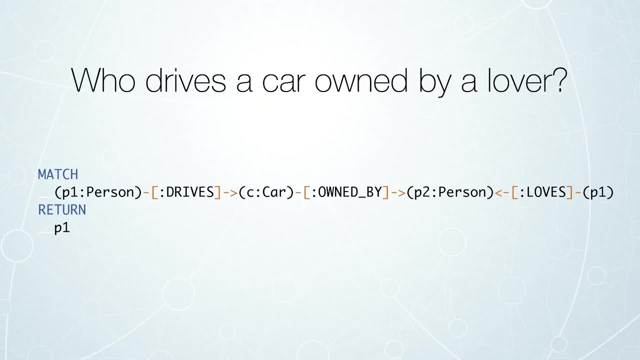 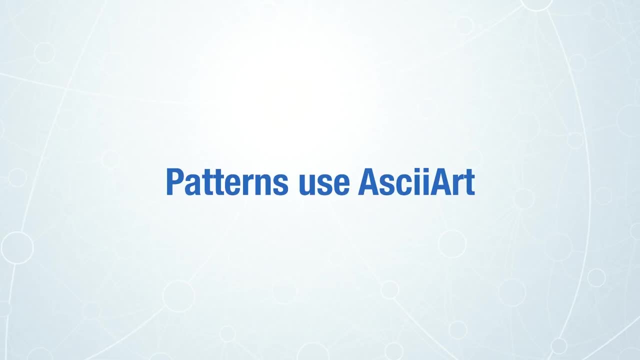 So really simple query to read and write, even though the question is a little bit more complex. Now, patterns in Cypher use ASCII art And, for those of you who weren't around back in the day, ASCII art is basically using the keys on the keyboard in order to generate graphics And in 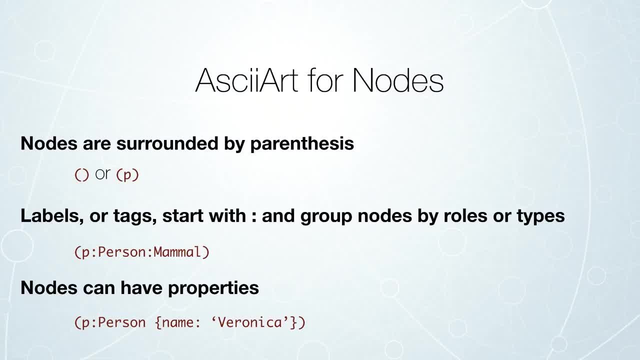 this case, ASCII art for nodes means that you're using parentheses to surround nodes And you can either just use a blank set of parentheses if you'll never need to refer to that node again after that part in the query, or you can specify an alias inside the node, such as P here in order. 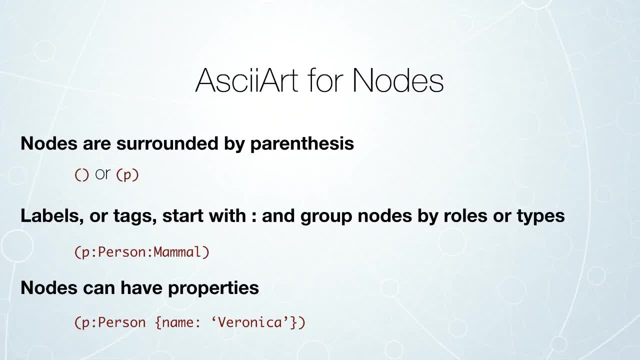 to refer to that node later in the query. There are also labels or tags on nodes. These allow you to group nodes together by roles and types. So in the case here of a person, a person is also a mammal. So this person has a second label that is a mammal. 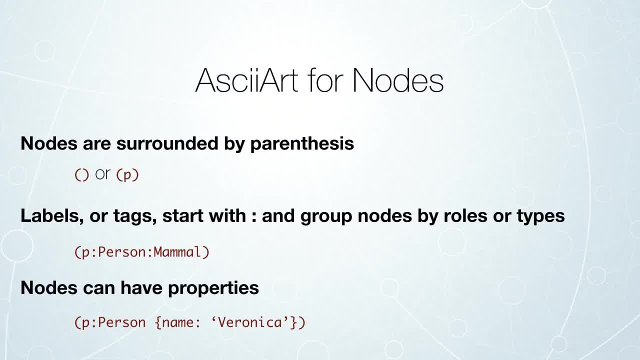 And we're going to still refer to that person as P as the alias. Now, nodes can also have properties, So, for instance, you might want to set the name on a person In this case. here we're setting the name on a person as the value string value: Veronica. The properties can have a wide variety. 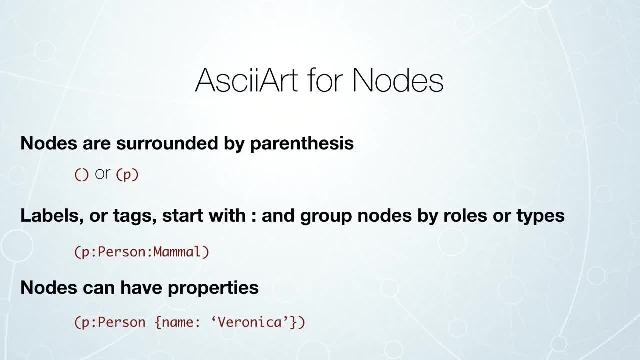 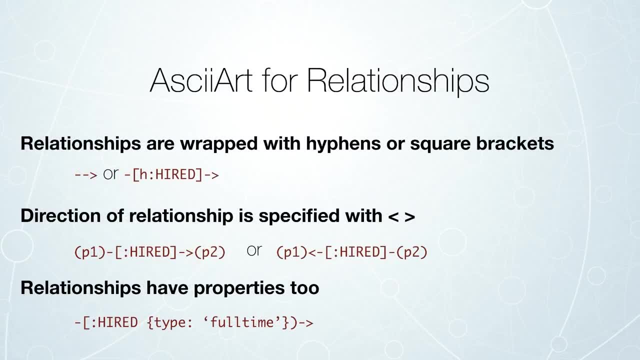 of different types of values, including a lot of the basic Java types and arrays of the basic types. ASCII art for relationships. well, relationships are wrapped with hyphens or square brackets. so you can see here, let's say, you were trying to talk about the hired relationships of Joe, hired John. you can see here that we could. 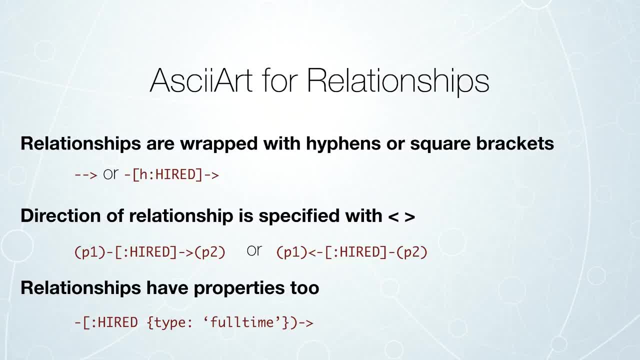 either specify the relationship- colon hired- with an alias H to refer to that relationship later in the query, or we could just say that there is a relationship without specifying the type and without specifying an alias. the direction of the relationship is specified with less than and greater than symbols. so you can see here person one, let's say Kate hired. person 2: 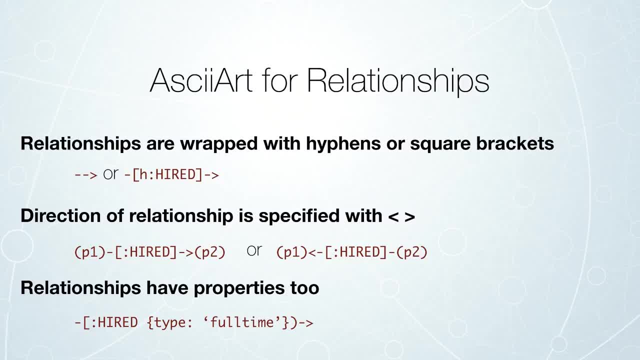 let's say John or the vice versa. and in the vice-versa case we have: Kate was hired by John or John Kate, but it's just showing the opposite direction, with the less than symbol instead of the greater than symbol. relationships can also have properties which can be specified using this JSON, like syntax, here in this case. 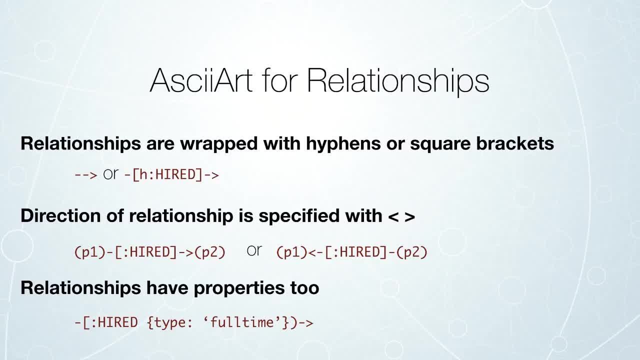 specifying that that person was hired as a type full-time employee. now I've mentioned the words aliases over time here and I want to re-emphasize this. so the H in hired here, the p1, the p2, these all represent references. so you're defining references or aliases such that later in the query you can access those. 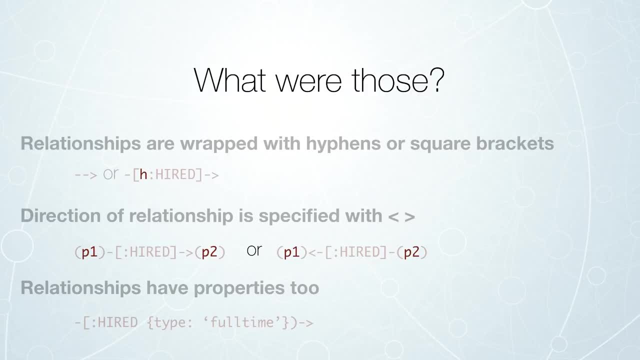 references. so in this case here, if these were in a match statement, we might want to return the person. you can access those references. so in this case here, if these were in a match statement, we might want to return the person back to the as a response to the query or if these were in a match statement. 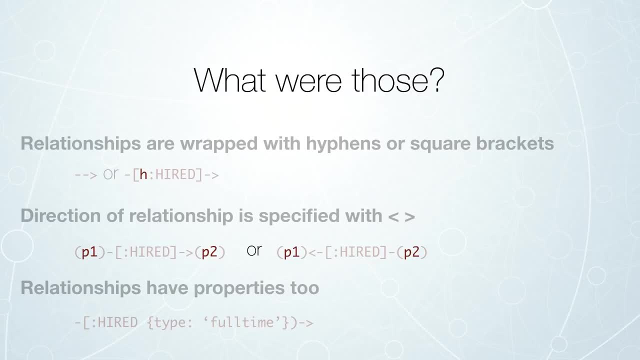 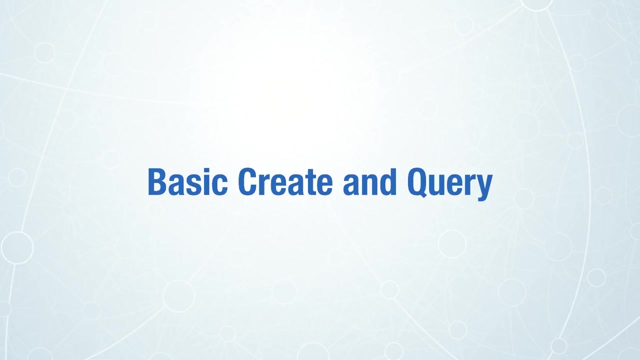 maybe we want to use that person that we found and we want to add additional properties or delete the person or something along those lines. so these are simply aliases that make it easier to access the match nodes or relationships later in the query. now let's give you a basic create statement, as well as a 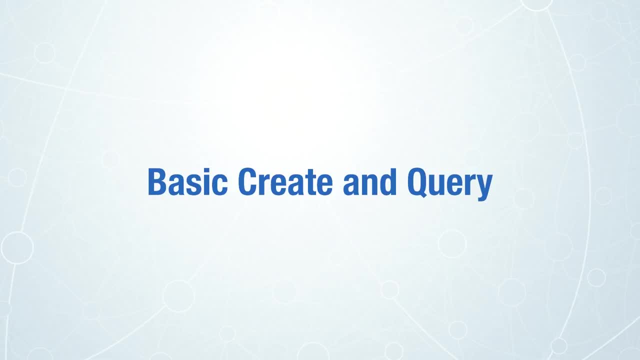 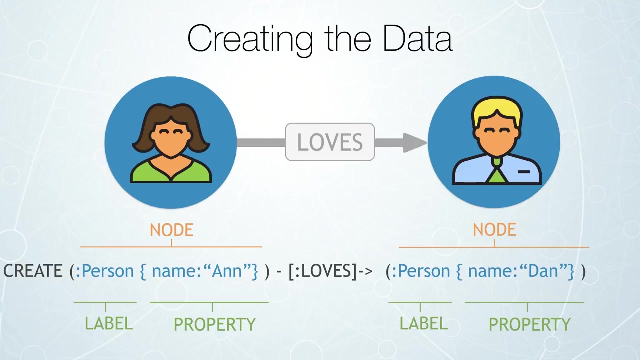 basic query statement. you know these are very simple examples here. later on we'll get more and more complex and we'll give you more complex query operations as well. to create data inside the graph, you simply specify it very much the same way as you would if you were trying to query for that data. so if 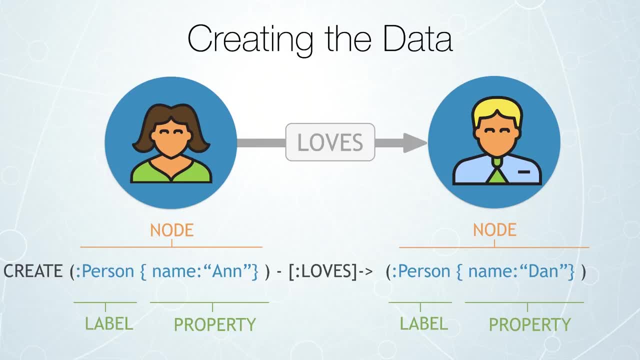 we wanted to create two nodes and a relationship between the nodes. in this case we wanted to create two person nodes as the label and have named properties on each of them and the loves relationship in between. we simply use the create statement in Cypher and we say: create colon, person brace and. 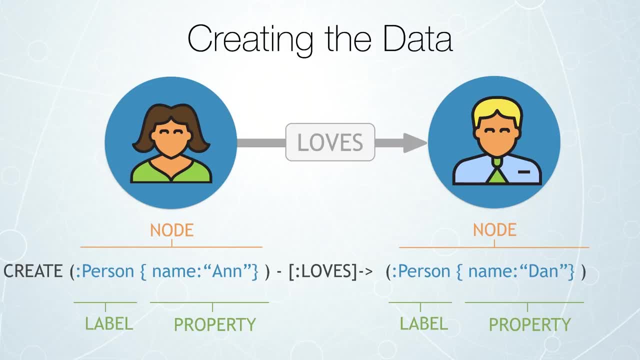 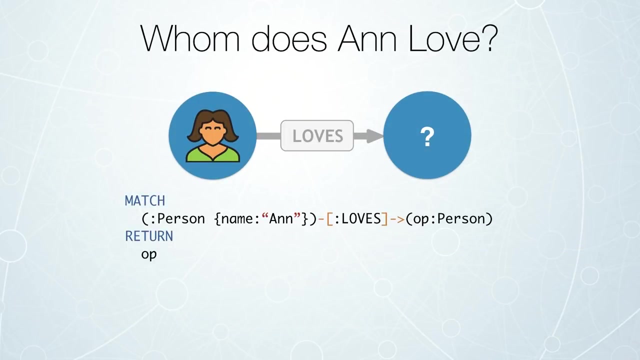 that JSON like syntax name and loves another person. brace in the JSON syntax name Dan, and that's all there really is to it. to it, This is all that it takes to create these two nodes and the corresponding relationship and the properties on the node in the graph. Now let's say we wanted to run a pretty basic. 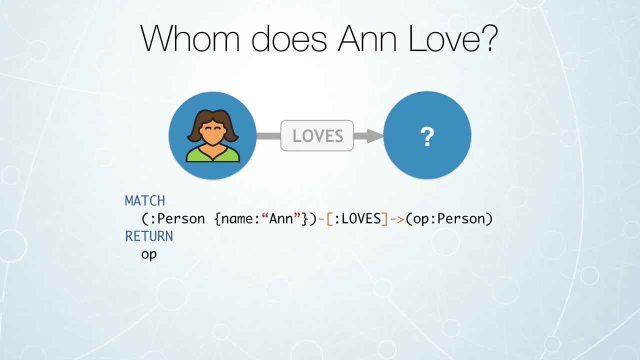 query and say, okay, we know Anne loves someone. Who does Anne love, Or whom does Anne love? And that query is actually quite simple. here We just say: find me a person named Anne who loves another person, And then you can see how we're using the alias here called op. 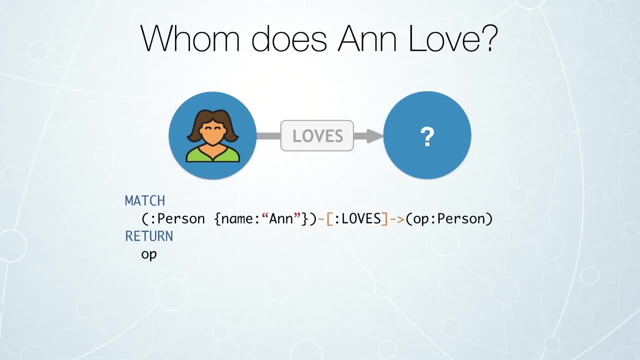 to return that other person back as a result of the query, And in this case we're returning the node and we get Dan, of course. So Anne loves Dan, And this is a really simple example here. It does show you the power of Cypher. What happens if we want to add more properties. 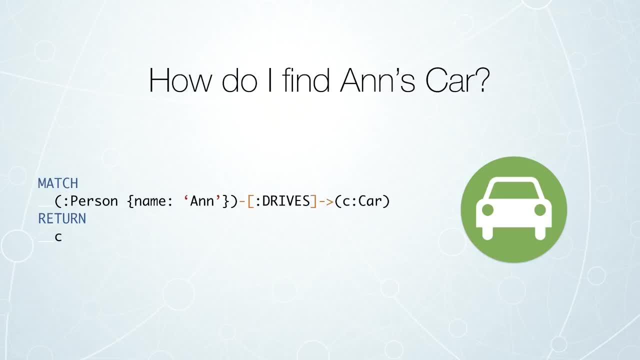 to our graph. Well, let's find Anne's car. We're going to find a person whose name is Anne- And you can see here I use single quotes. here, when specifying Anne, You can use either single quotes or double quotes- And let's find a person whose name is Anne who drives. 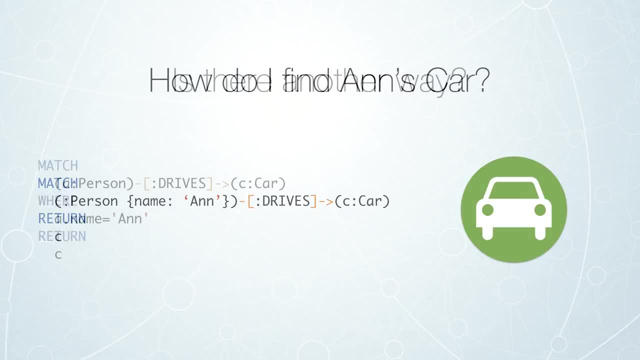 a car And let's figure out the car that Anne drives. We can actually do this in another way. The first example was using the JSON-like syntax for specifying the name of the person that we're searching for. In this case, we're actually. 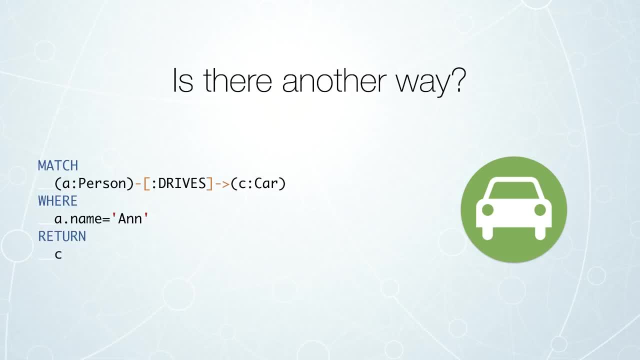 just saying that the pattern that we're searching for is a person who drives a car, And then we're restricting the traversal by specifying the name as Anne. Both of these queries should really have the same performance, But you know, different ones are more readable than others by different people, So take those two different options. 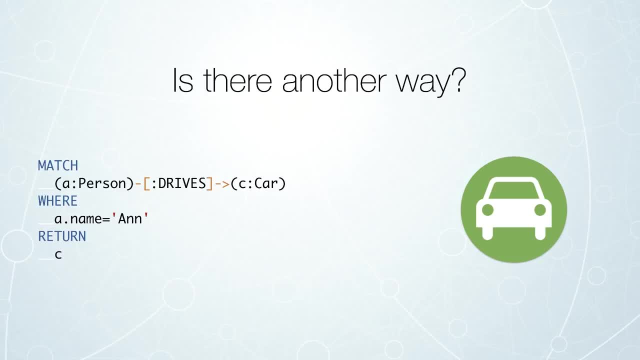 and understand that they mean the same thing. But in this case we're returning the car that Anne drives. Now let's say we wanted to add greater description to that car. We wanted to indicate the brand and the model of the car. We can easily do that with the set operation, So the set syntax. 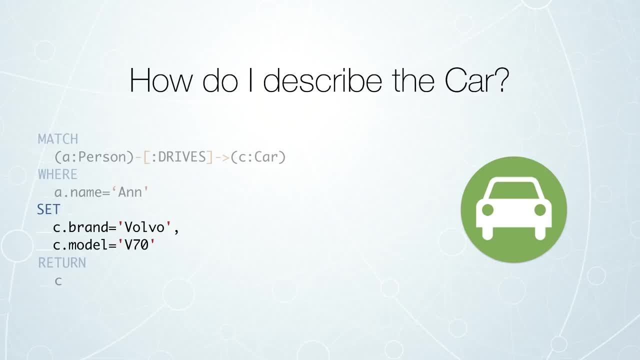 in Cypher. It allows us to set additional properties on the node that we found. So it's the same match statement. We're trying to find in the graph a person who drives a car where the person's name is Anne, And we're also trying to return that car, But here, before we return, 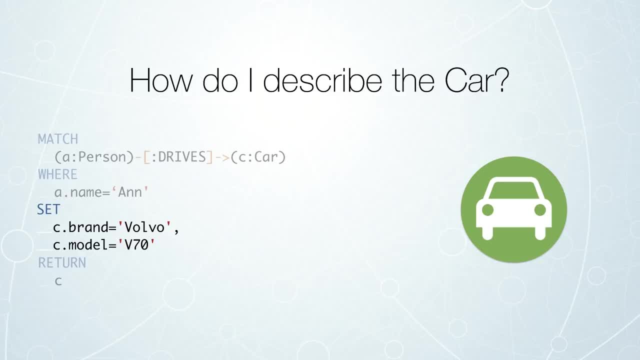 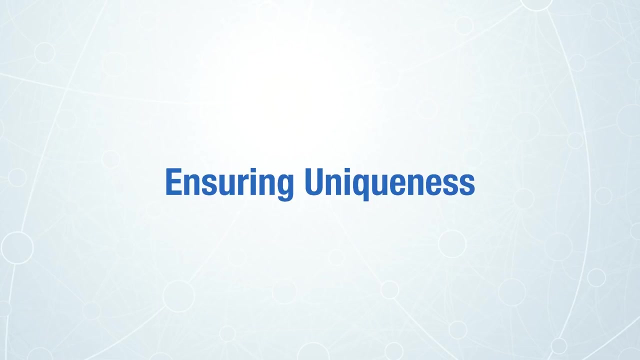 it. we're going to set those two additional properties- the brand and the model- And then the returned car will have those properties set. One important aspect of dealing with graphs is dealing with the integrity of the graph, the integrity of the data, And Neo4j really focuses on being a transactional database. 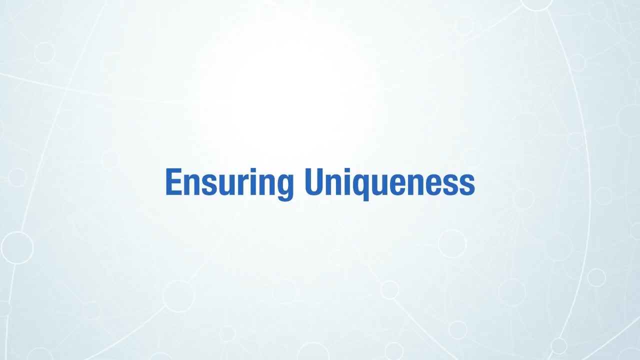 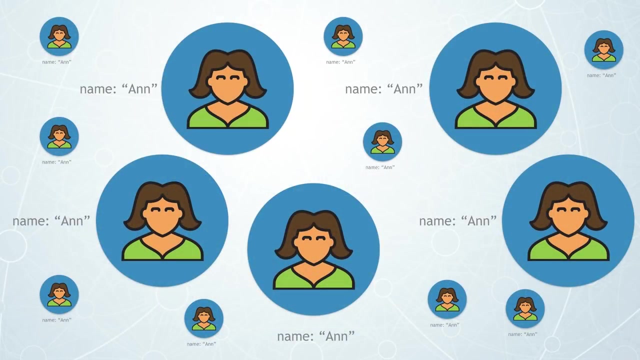 OLTP has ACID compliance. We're all about making sure that the data that you set and the data that you return is all predictable, And one of the aspects of that is in terms of ensuring uniqueness in the graph. We don't want you to have a bunch of different. 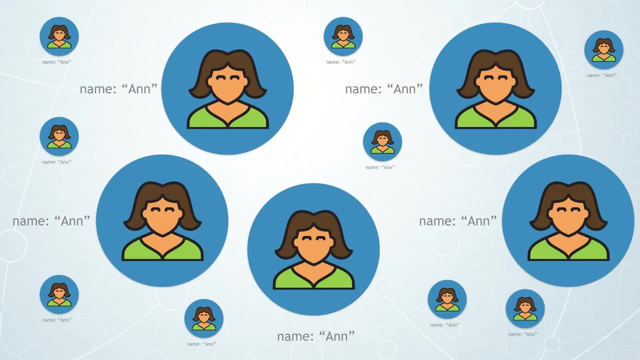 Annes in your graph. Let's say that your graph looked like this: how would you know how to differentiate one Anne from another Anne? That would be very difficult. So we're going to assume here that the name Anne is unique amongst the population in our graph. We can 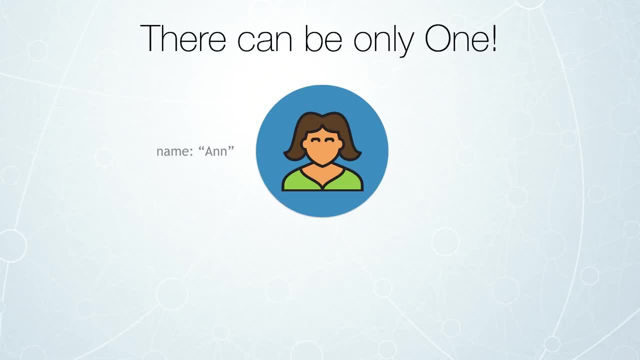 actually ensure that there can only be one, Anne. We can do that with constraints. In this case. here we're going to say: create constraint on the person. labeled nodes assert that the person's name is unique. it's a very simple constraint, but it's very powerful to prevent us from adding multiple ands. so let's say we did try to. 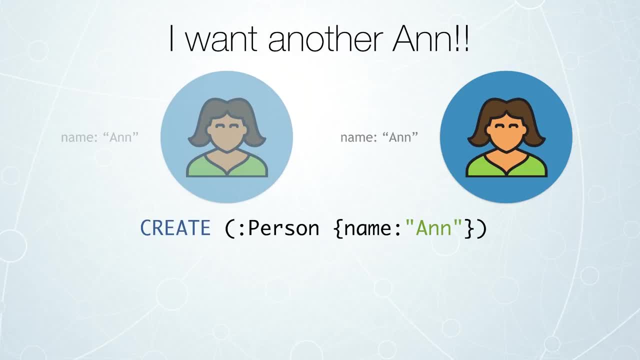 add another. and if we tried to add another and by creating another person labeled node with a name of an, we would actually get an error that looks something like this: constraint validation failed, indicating that there's another node in our graph already with the same label and the same property, and that violates our constraint that we set. 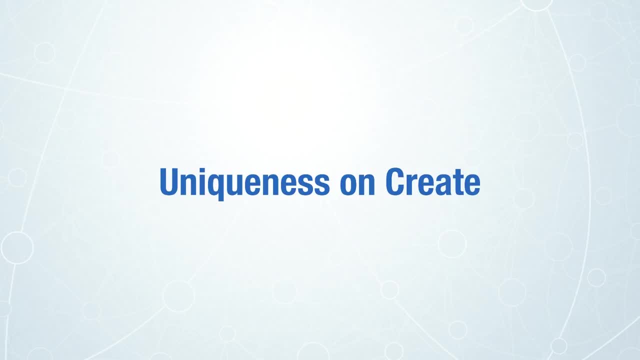 of course, this is all fine and dandy, but we don't want to actually experience this error. we want to actually be able to ensure you need to have a constraint that is unique, and that's what we're going to do. we're going to create a constraint that is unique, and that's what we're going to do. 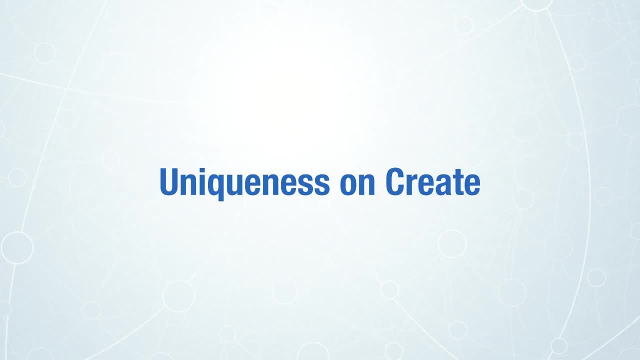 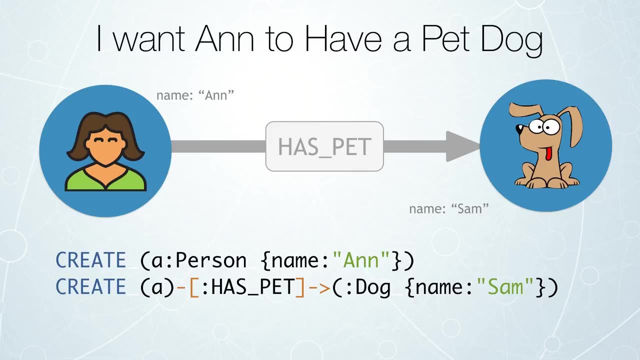 we're going to create a constraint that is unique and that's what we're going to do, this at the time that we create our nodes and relationships. so let's say that we want anne to have a pet dog. so we want to say anne has pet and named sam. if we did something like this, 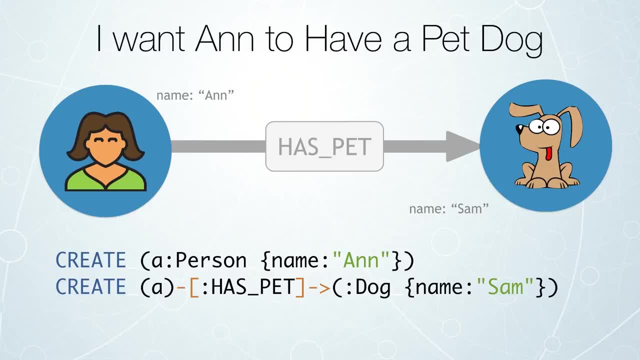 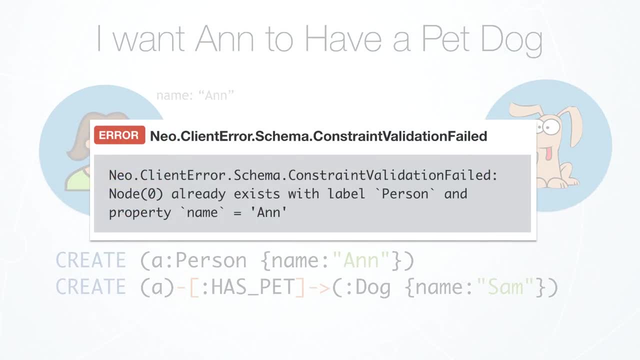 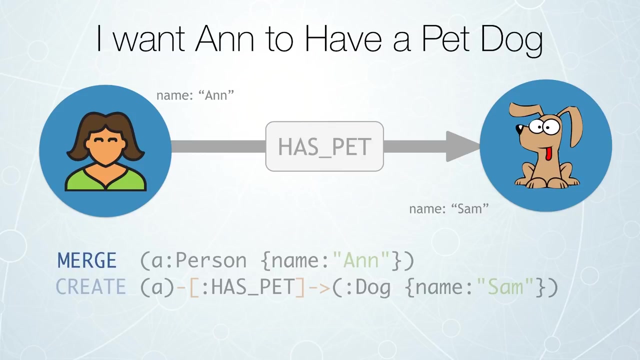 create a person named anne. create a. has a pet dog named sam. we'd actually experience the same error as we talked about before: a constraint validation error, because anne already exists in our database. so instead of using to create statements here, we can instead use a merge statement and saying: merge- person named anne. 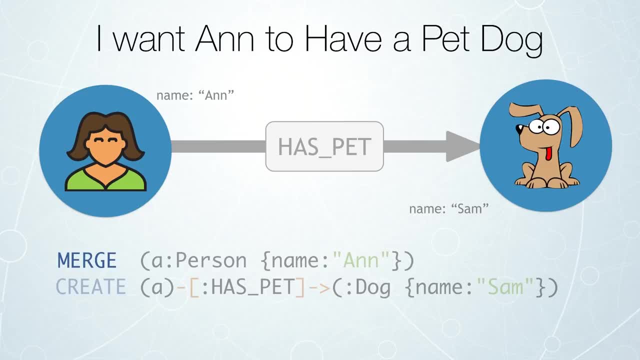 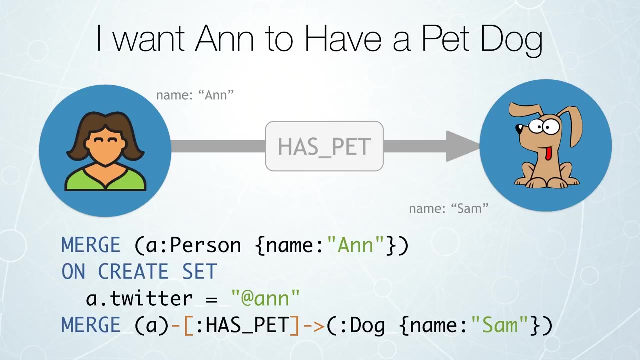 basically what this does is it looks in the graph for a person named anne and operates on that person node if it exists. if it does not exist, it will create it and that way, when you execute the next step in terms of creating the relationships, you can create that dog attached to either the existing person or a new person, in this case here.